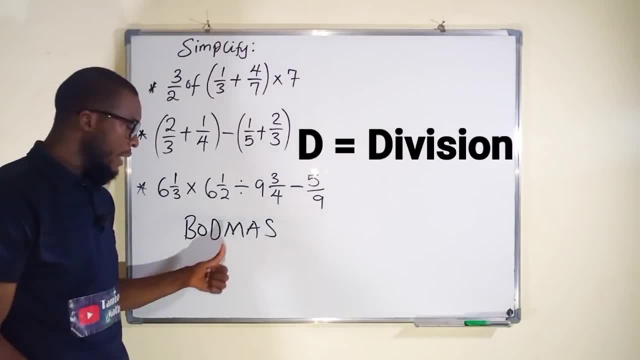 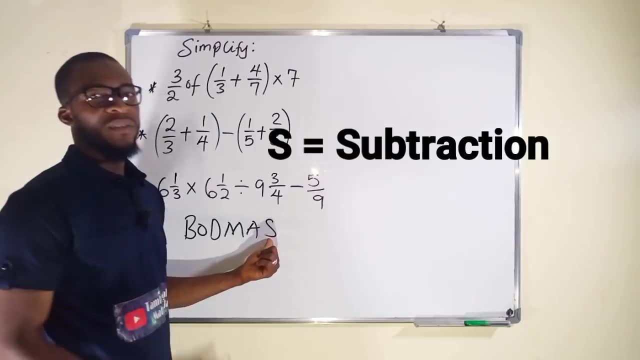 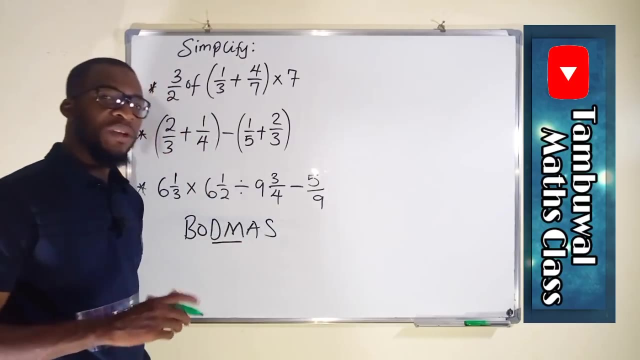 orders. D stands for division, M stands for multiplication, A stands for addition And S stands for subtraction. But the rule said division and multiplication are done simultaneously from the left to right, starting with the one that comes first. If you see multiplication before division. 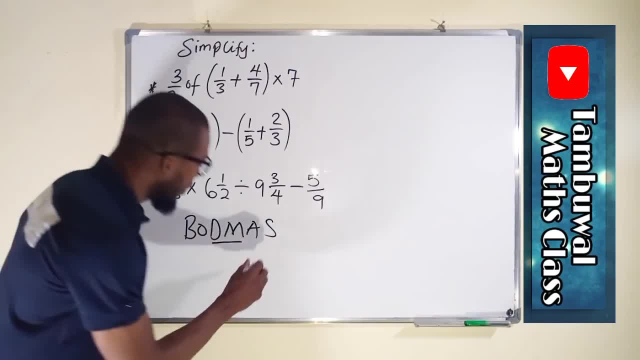 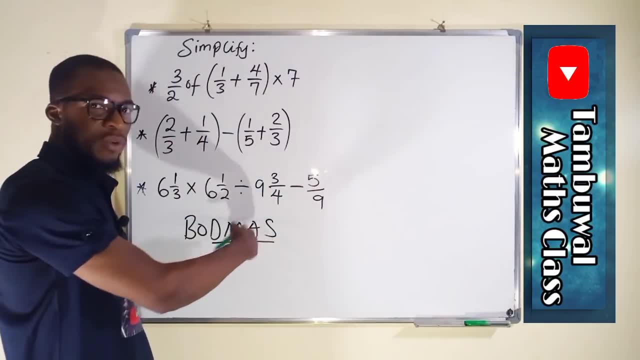 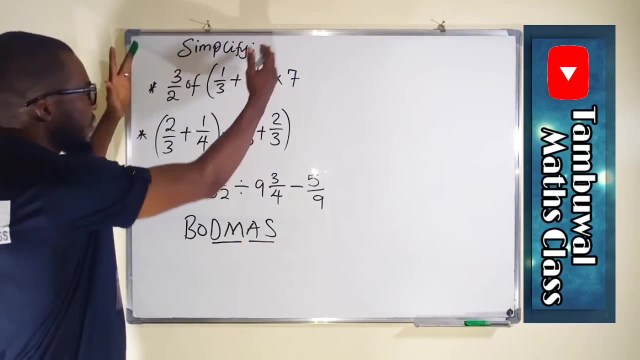 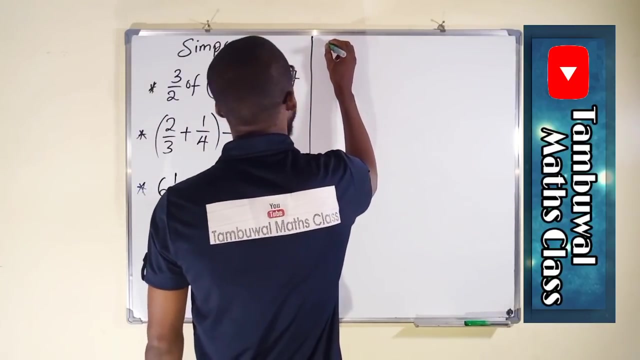 you start with multiplication and vice versa. The same thing: addition and subtraction are done simultaneously, from left to right, starting with anyone that comes first. If you see subtraction before addition, you begin with subtraction and vice versa. So now let us begin with this. 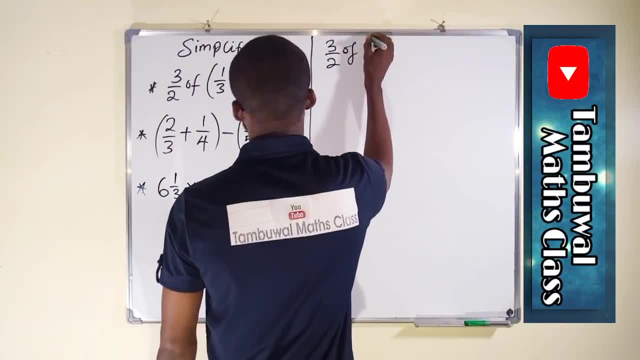 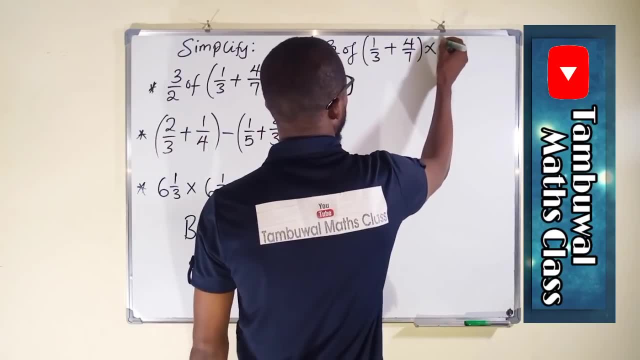 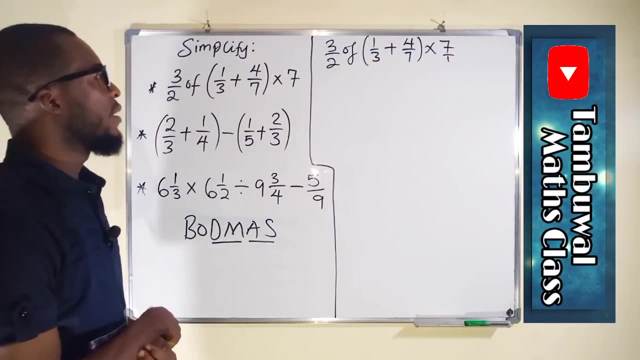 We have 3 over 2, of 1 over 3, plus 4 over 7 times 7.. We can even rationalize this 7 as 7 over 1, because 7 over 1 is still 7.. Following this rule: 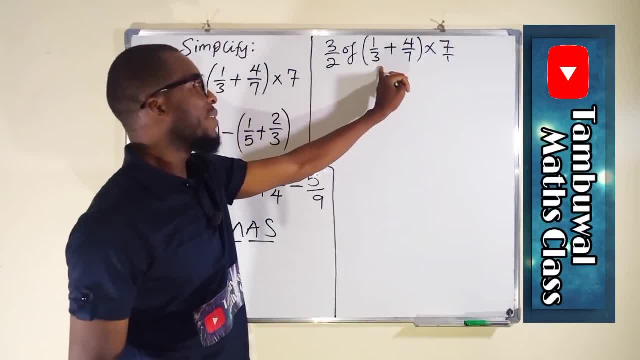 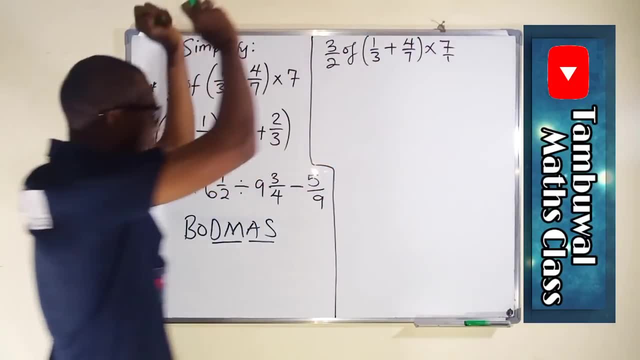 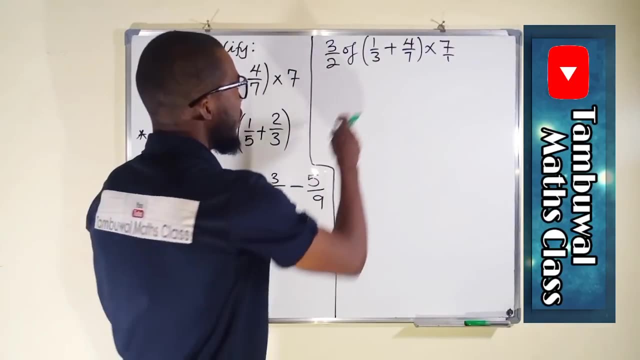 we have bracket. Therefore we have to begin with 1 over 3 plus 4 over 7, because there are diffractions under the bracket. So first, this bracket is absent. here We have to begin with orders which we have off as part of orders. Okay, These fractions have different. 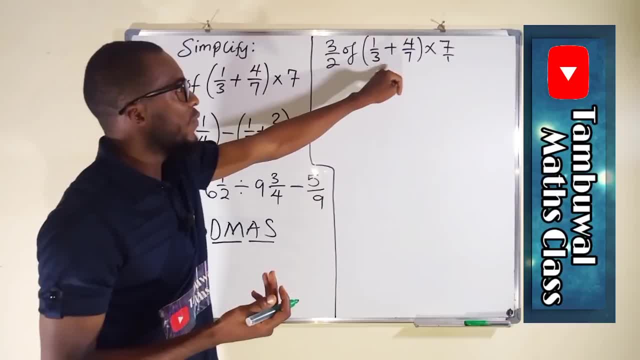 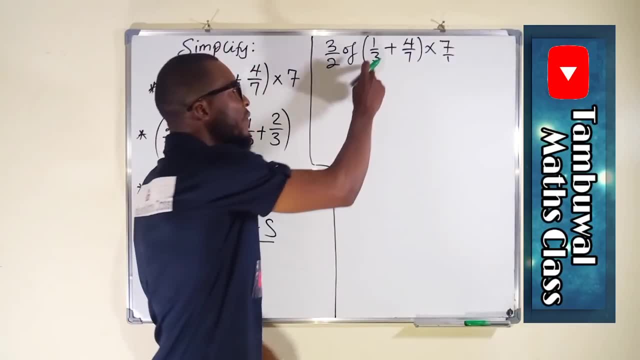 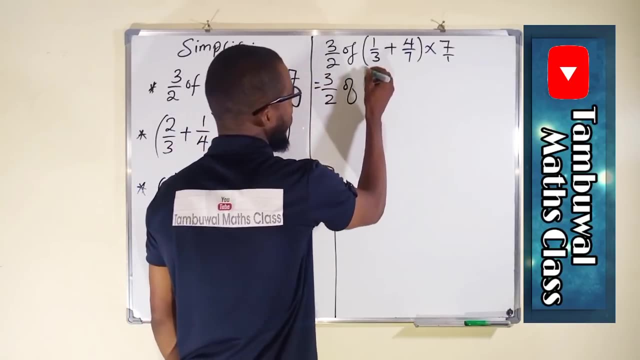 denominators. For convenience, let us transform them in such a way they will have the same denominator And the LCM of these 3 and 7 is 21.. So we are going to convert them into 21.. So we have 3 over 2 of to change this into 21,. we have to multiply it by 7.. For 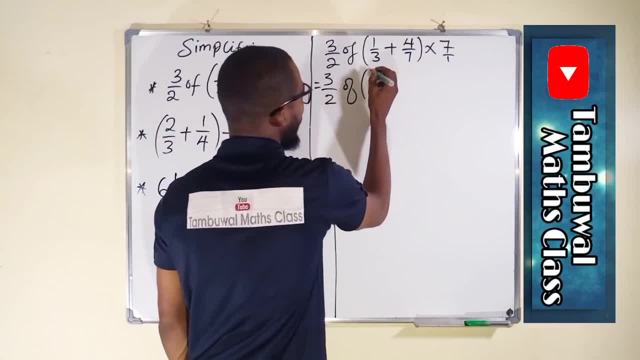 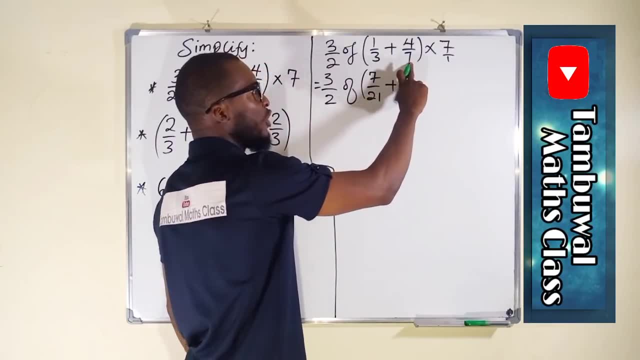 equivalency. we have to multiply the top number by the same value. 7 times 1 is 7.. 7 times 3 is 21.. Plus, to change this into 21, we have to multiply it by 3. And we have. 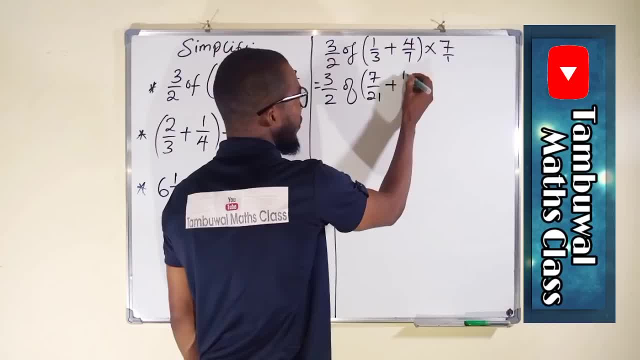 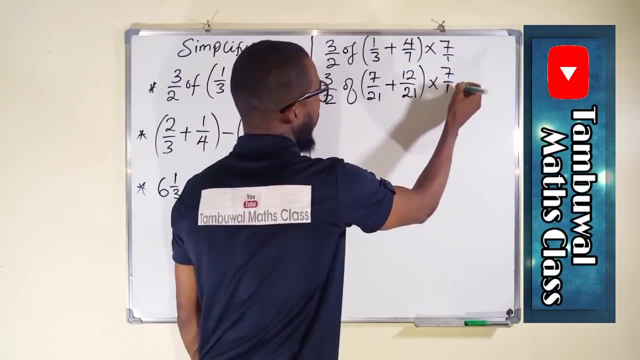 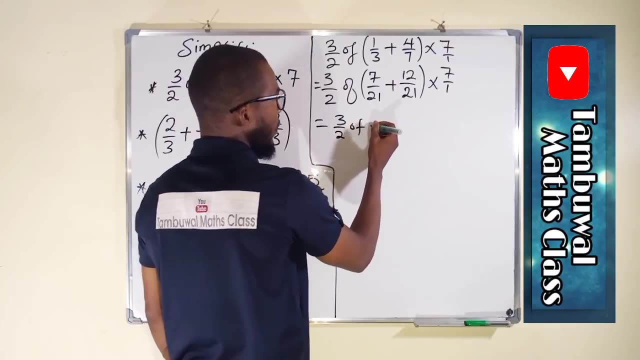 to do the same to the top number. 4 times 3 is 12.. Over 21.. Multiply by 7 over 1. This is equal to 3 over 2 of 7 plus 12 is 19.. So this is 7 times 3, is 21 plus We have. 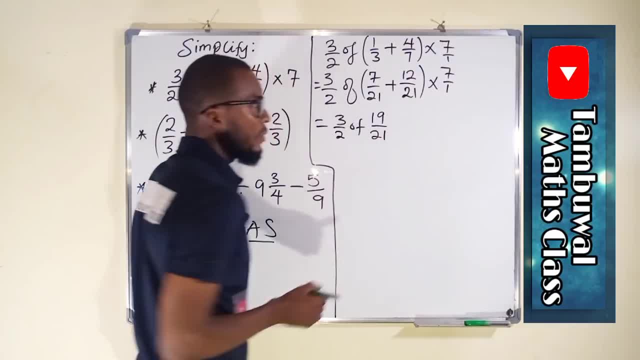 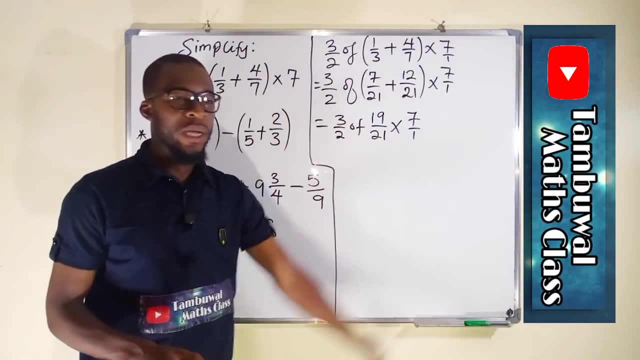 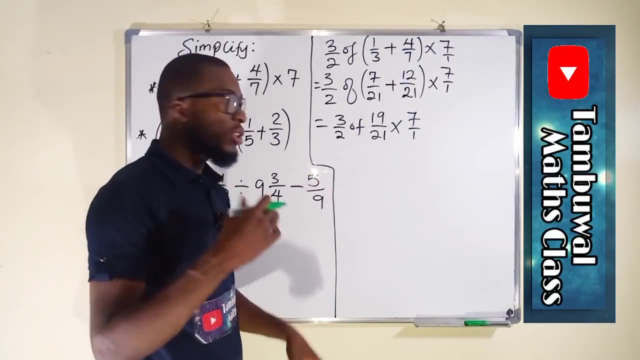 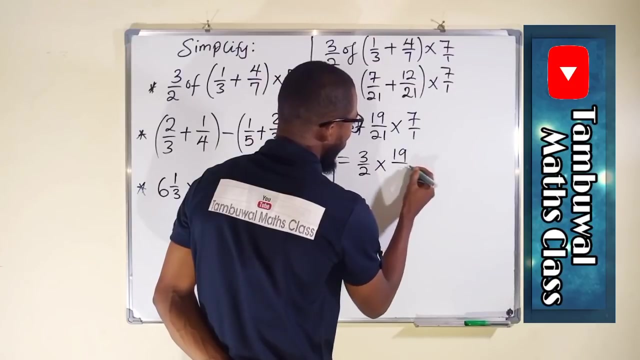 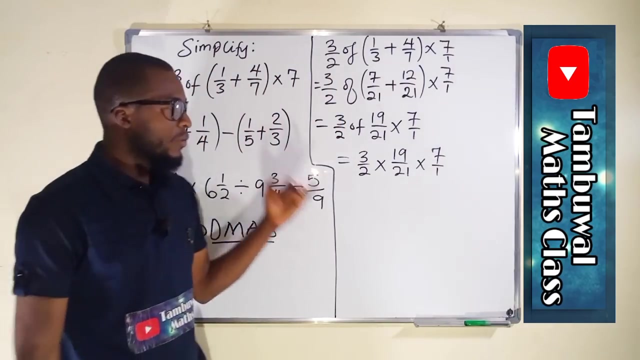 over 21 times 7 over 1. we have cleared the bracket. then we move to the next one order. we have off here, and this off is the same thing as multiplication. so this becomes 3 over 2 multiplied by 19 over 21, multiplied by 7 over 1. so you can see. 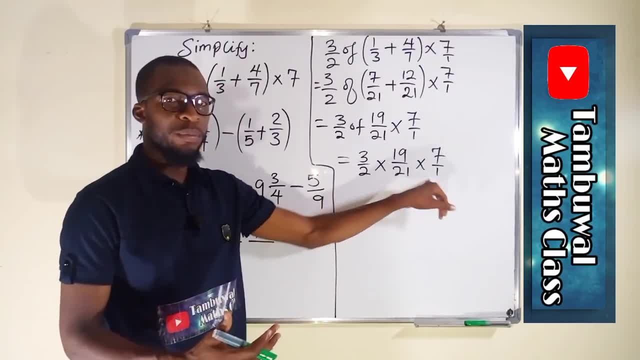 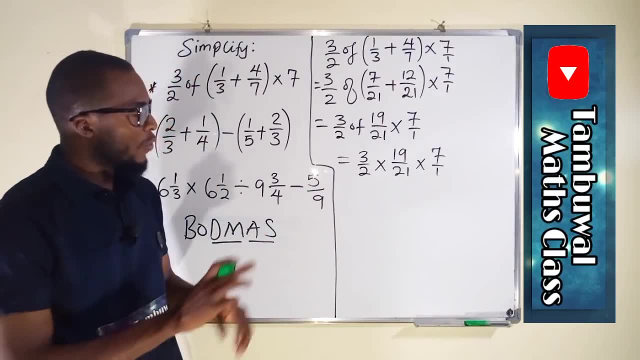 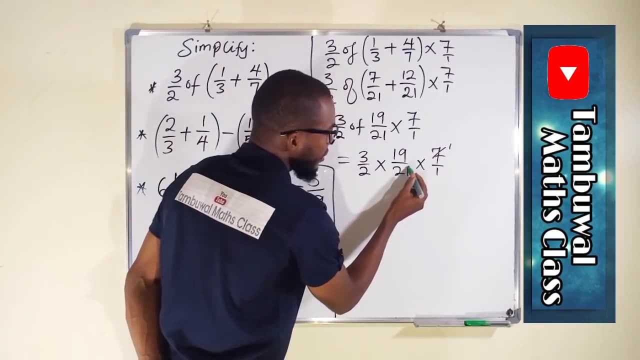 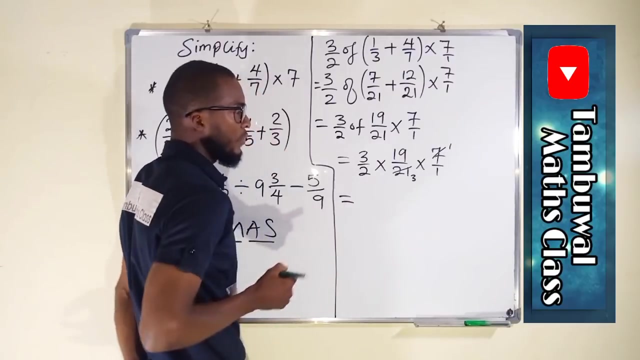 the operations we have left. they are of the same kind, multiplication, so we can just multiply the top numbers and the bottom numbers separately, but for convenience let us reduce them to their lowest times. you can see 7 here. I can go into 7 12 time and 7 can go into 21 three times. so this is equal to 3 times 19 is 57, 57. 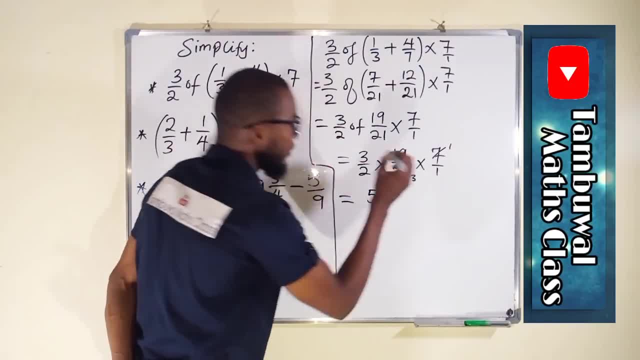 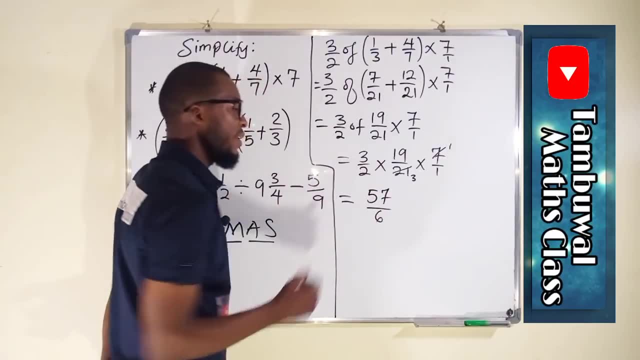 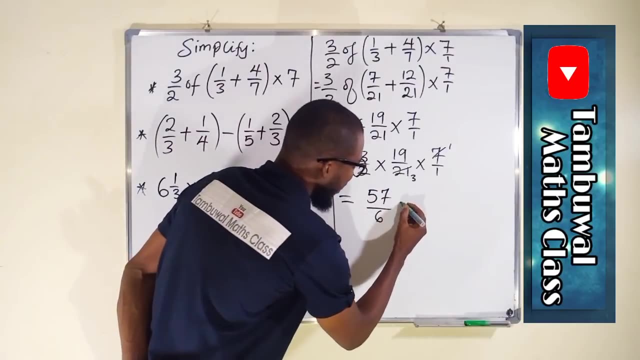 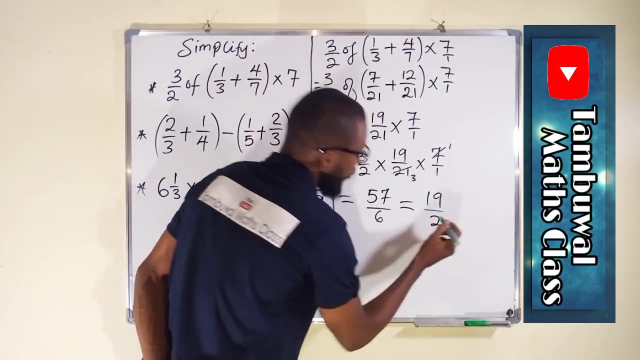 times 1 is still 57. here we have 2 times 3, which is equal to 6. so now let us reduce it to the lowest time: 57 divided by 2 times 3, which is equal to X. the lowest, then, 6, divided by 3, is 19. 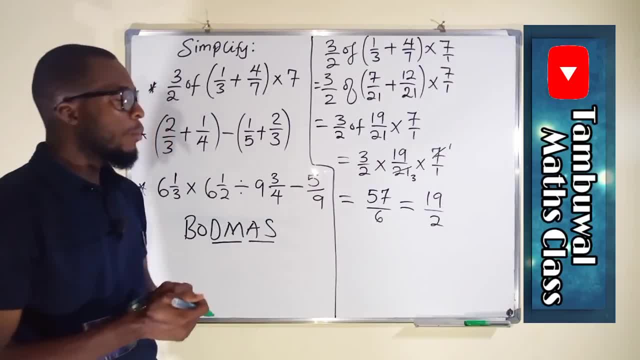 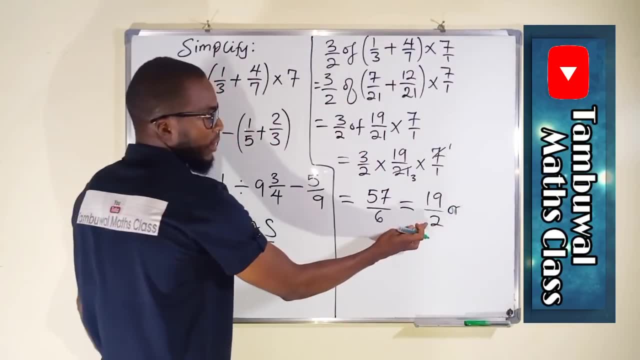 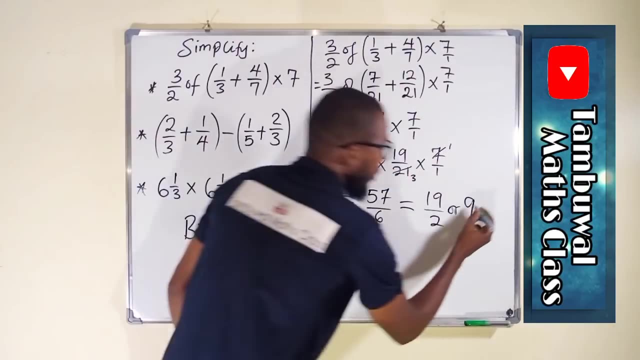 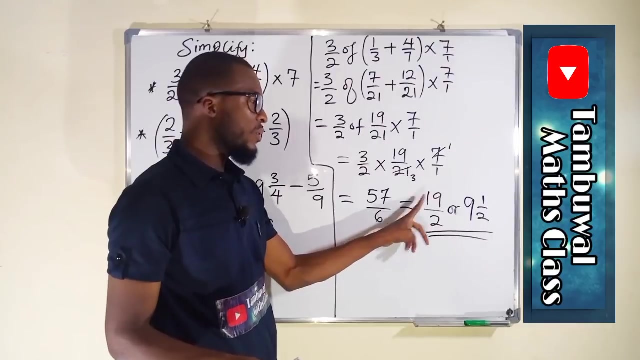 then 6 divided by 3 is 2. this is our final answer, because nineteen and two do not have any common factor, but still we can reduce it into a mixed number. therefore we can see: O two can go into twenty nine times out of two. so this, either this or this. this is an improper fraction. this is in mixed number. 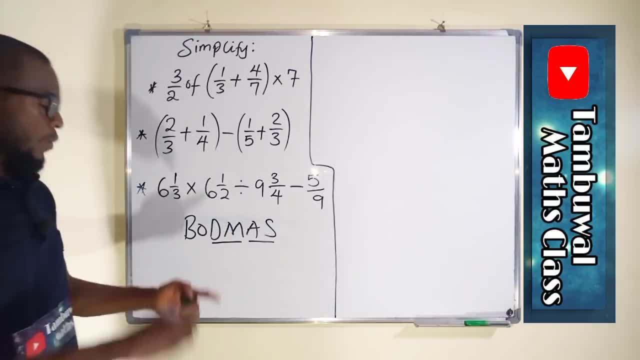 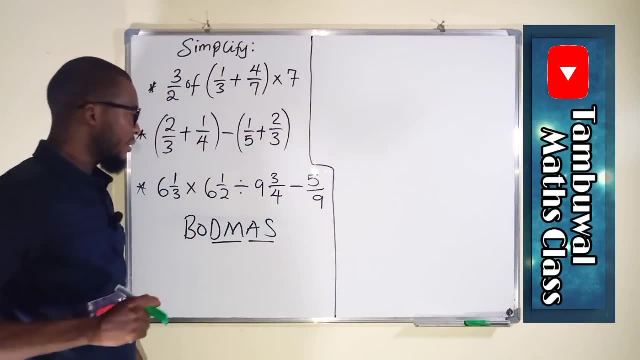 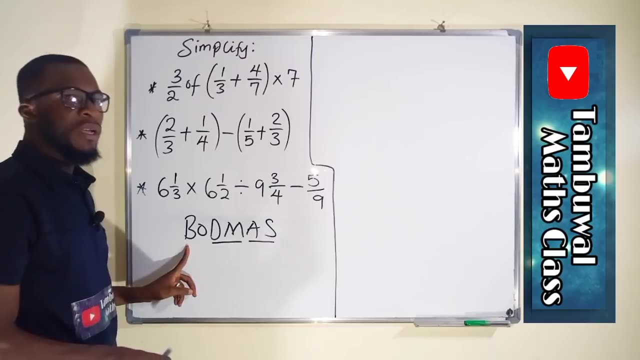 let us move on to the next one, the next question. you can see we have two brackets separated by a negative sign. so it means we are going to subtract the whole of this bundle from this. but all of them are brackets because we have bracket first. so bracket doesn't specify whether we should start from the right. 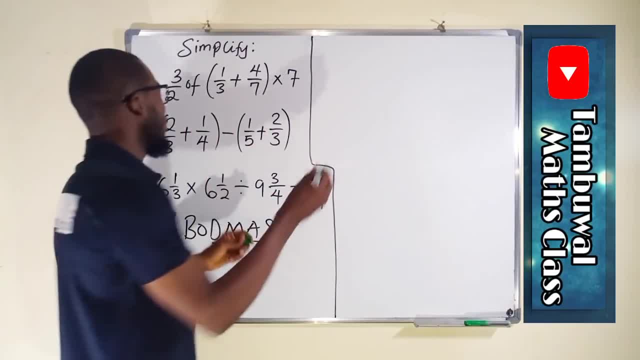 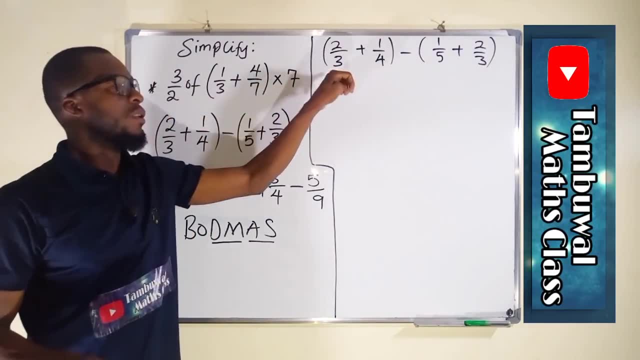 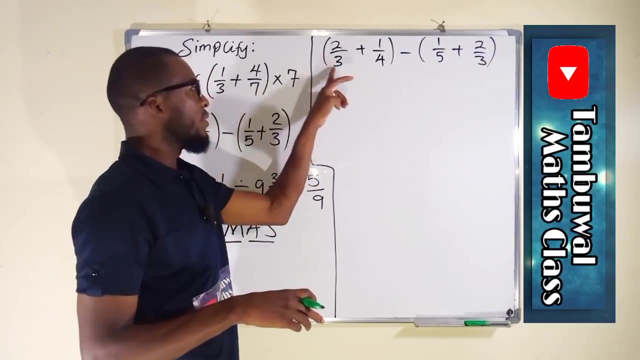 bracket or the left bracket. we can do them simultaneously, so we have two. let us convert their denominators into the same value. the lcm of three and four is twelve, because twelve is the smallest number in which three and four can go into without remainder. so to change this into twelve, you have to multiply it by four. 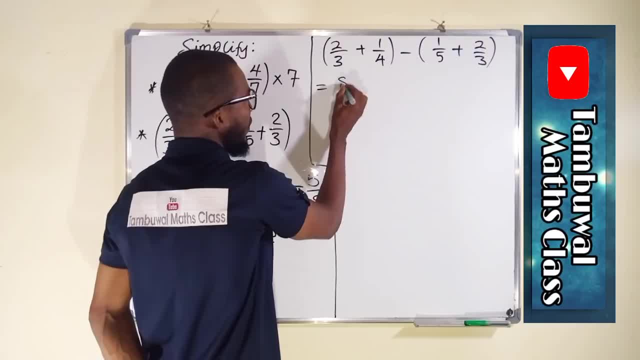 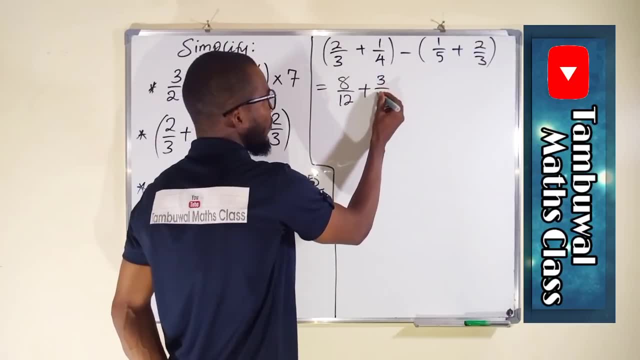 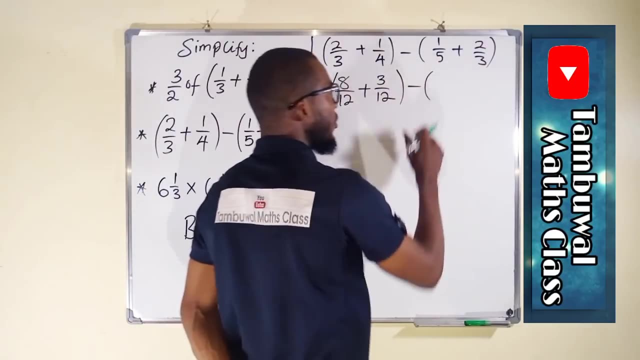 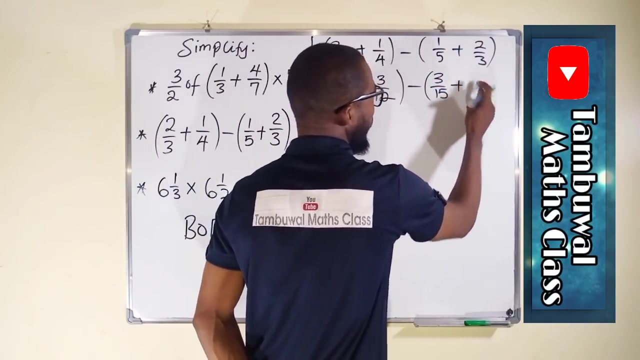 you have to do the same to the top number. four times two is eight. four times three is twelve. three times one is three. three times four is twelve. the lcm here is fifteen. to change five into fifteen, you multiply it by three. do the same to the top number, three over fifteen plus to change this to fifteen multiplied by five. do 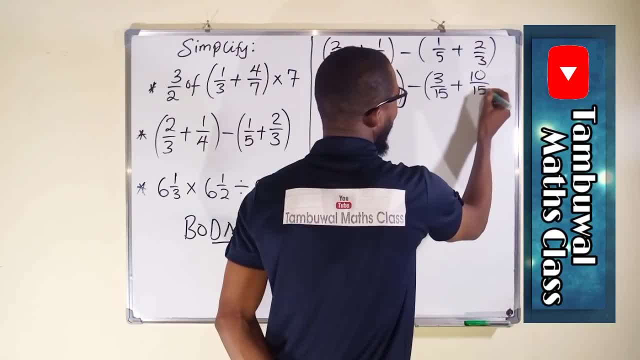 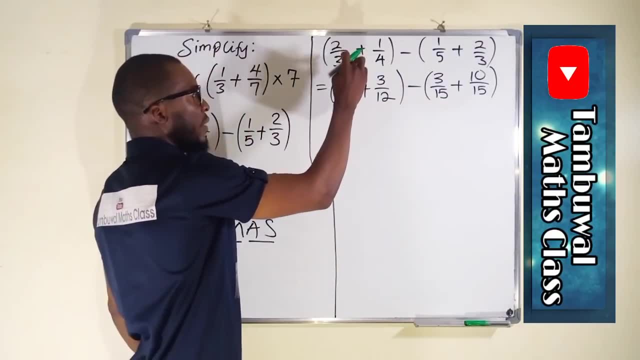 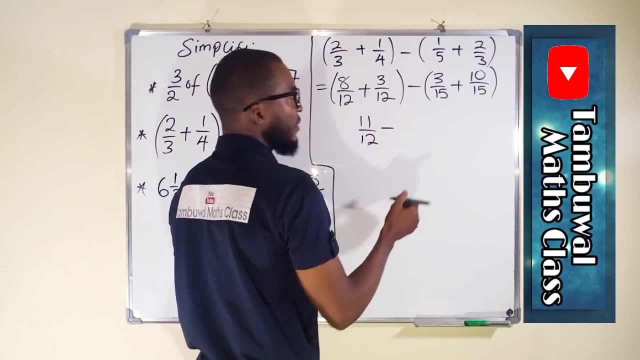 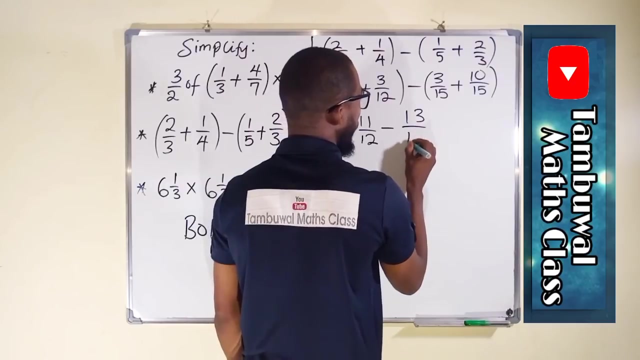 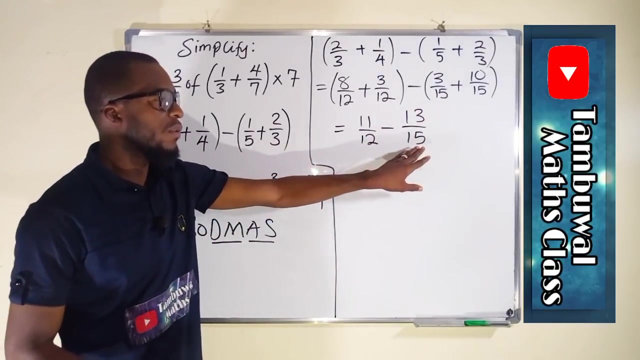 the same to the top number, because five times two is ten, so we are not free to simplify these brackets. this plus this is 11, so we have 11 out of 12. minus this plus this is 13 out of 15.. so this is what we have left. we want to subtract 13 over 15. 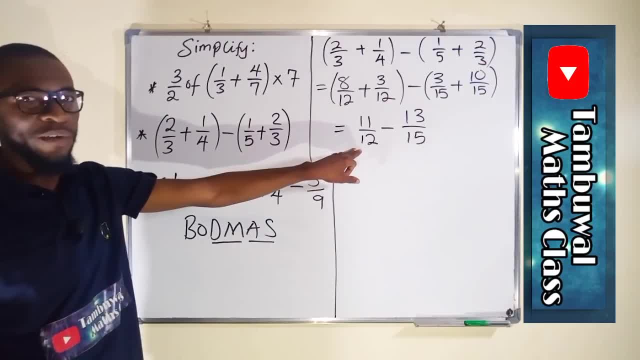 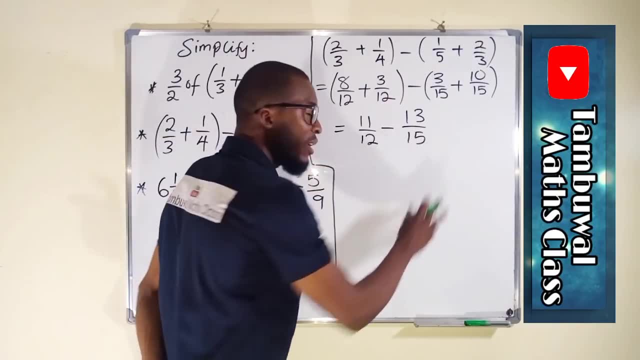 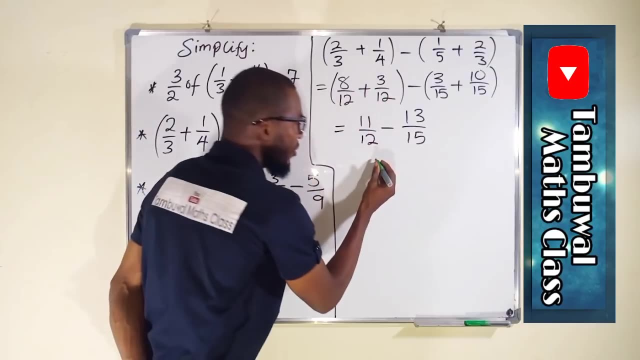 so we have one half needs 11 over 14, which is 15, and so the final pass is 16 and 15 out of 11 over 12. let us convert them into the same denominator, um. let us change them into 60.. to change this one into 60, you have to. 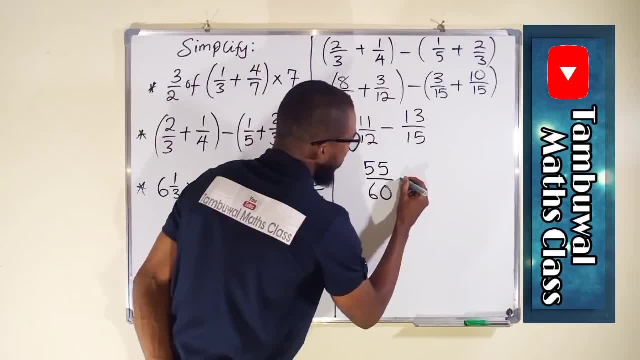 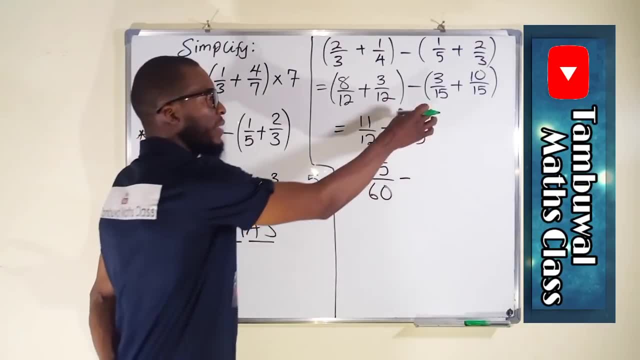 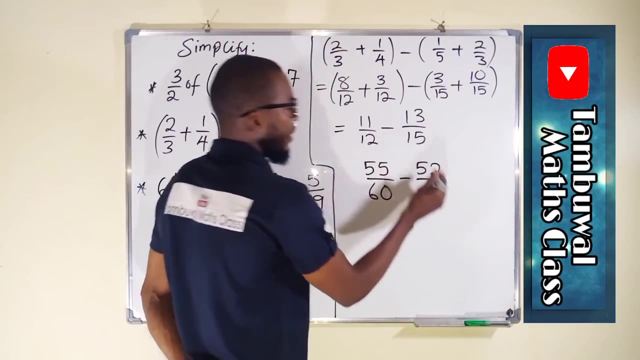 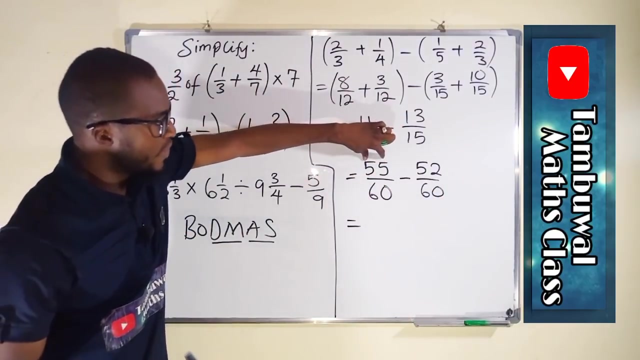 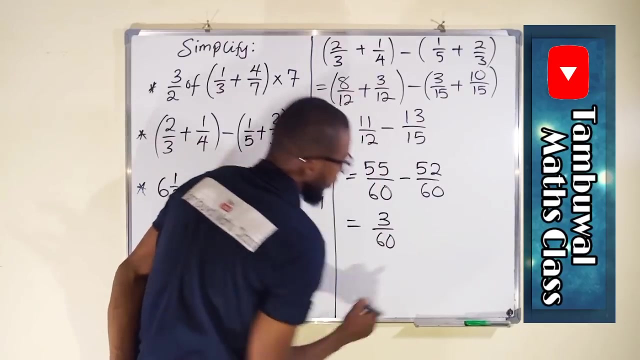 multiply it by five. we have to do the same to the top number. 11 times 5 is 55 over 60, 4 is 52 and this times 4 is 60. this is equal to 55 minus 52 is 3 out of 60. but 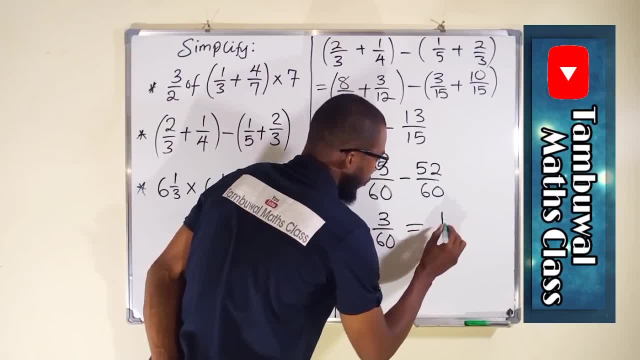 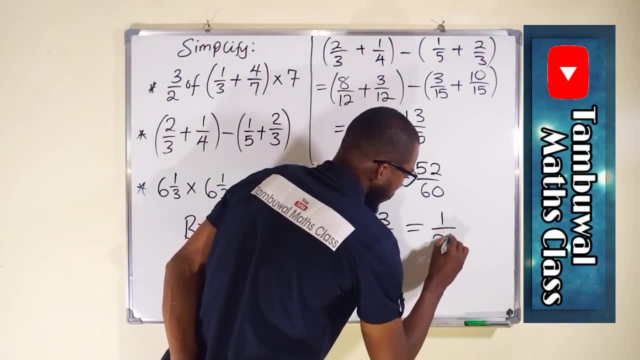 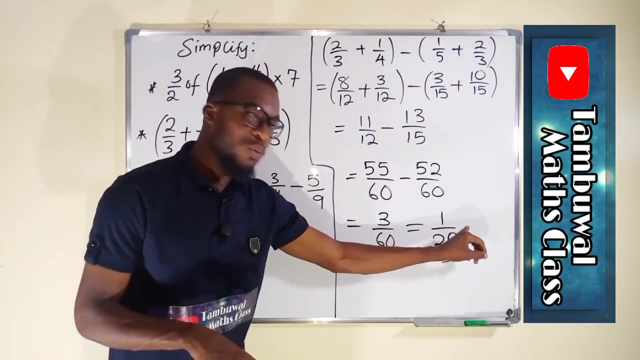 3 can go into 3 one time, so we can reduce this one, and 3 as well, can go into 60 20 times. so our final answer is 1 over 20, because you cannot reduce this one into a mixed number, because this is a proper fraction. remember, you can only. 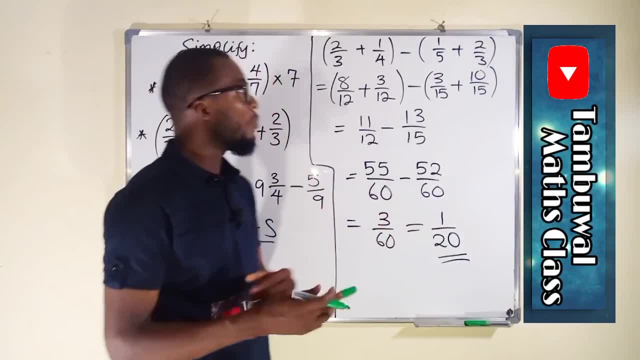 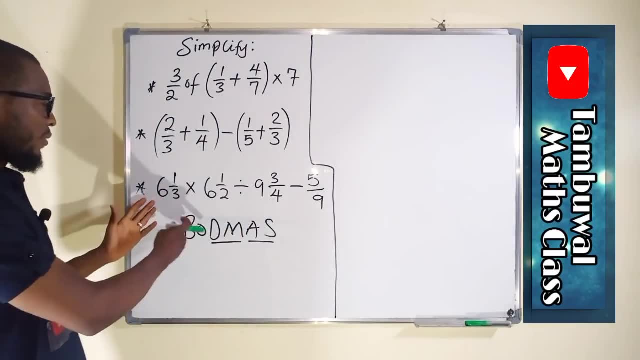 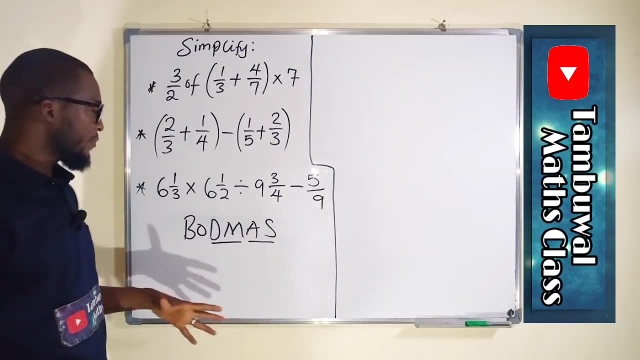 convert improper fraction into a mixed number. so now let us take the last one. so here is the last one. you see, we have combination of mixed numbers and a fraction using the same principle of Bode mass. we have to start with bracket, which is absent here. orders is also absent. division and multiplication. 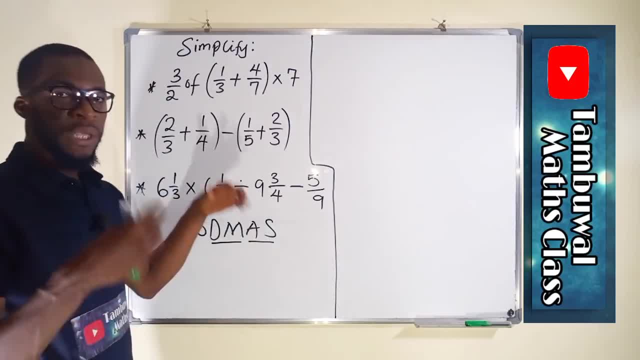 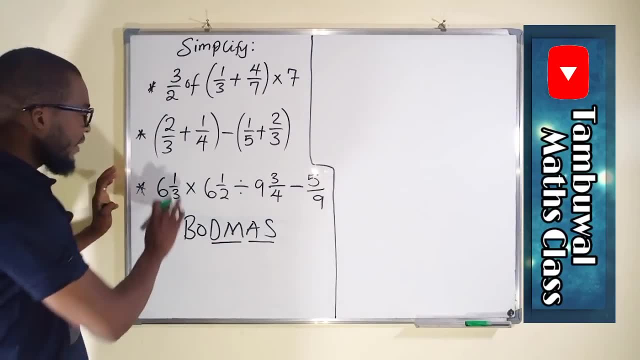 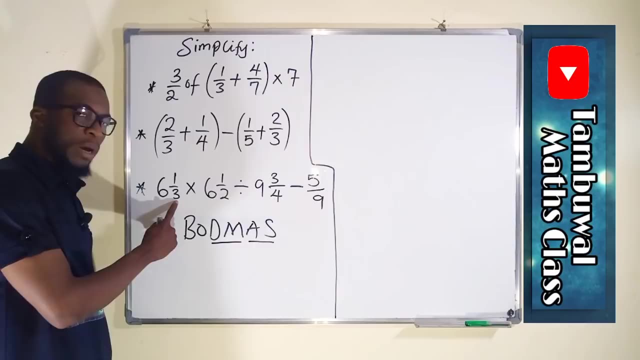 you see, we have multiplication and division. I told you, you always start with the one that comes first. and lastly, you see, we have subtraction. but for convenience, let us transform these mixed numbers into improper fractions. you take a fraction in an order to substitute not just one but also the other, and 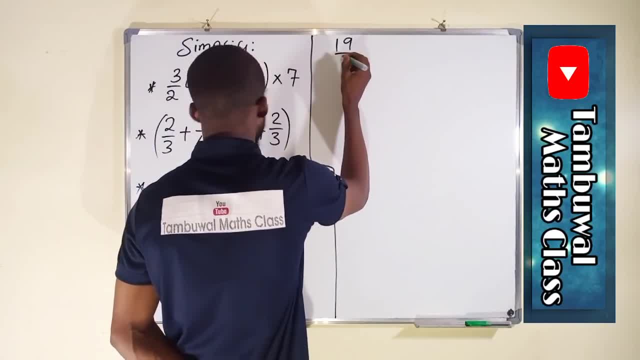 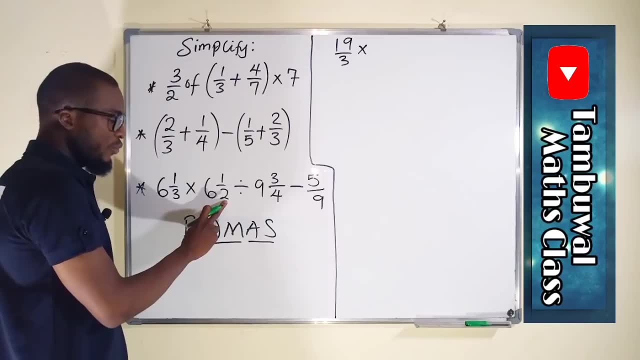 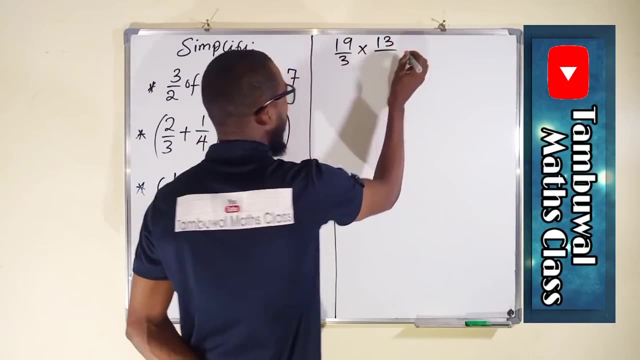 now we are going to say a multiplication of mixed numbers, say Y, Y, 2, a and aobilion a and a, lippar a, b and the set of transactions plus change to data- somewhat of the same process. you can use it again. you can take a multiplication and divide it into a. 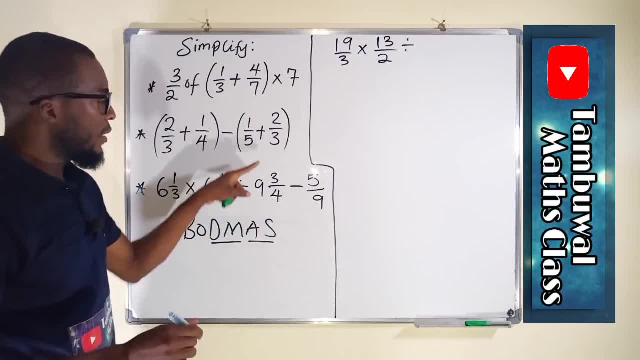 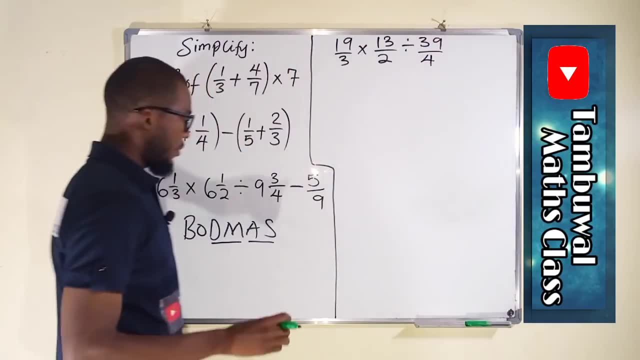 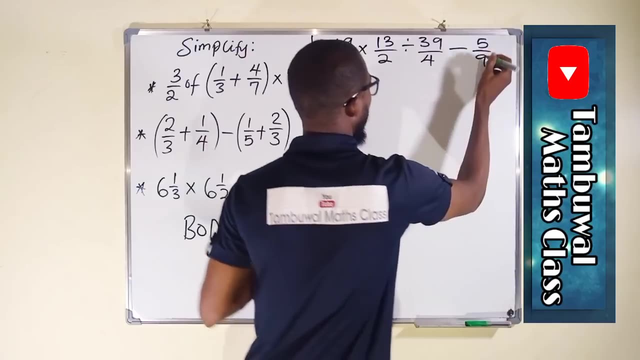 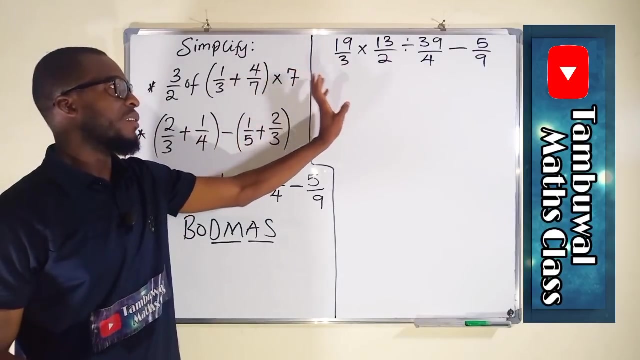 4 times 9 is 36.. 36 plus 3 is 39. So we have 39 over 4.. And the last one minus 5 over 9.. So from the rules, division and multiplication are done simultaneously from left to right. 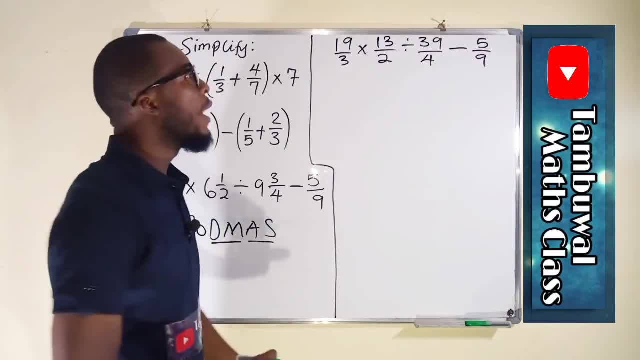 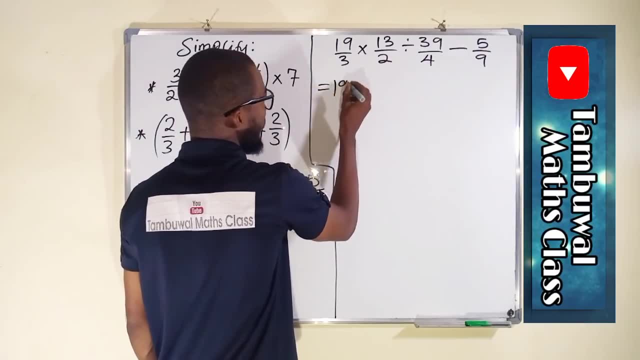 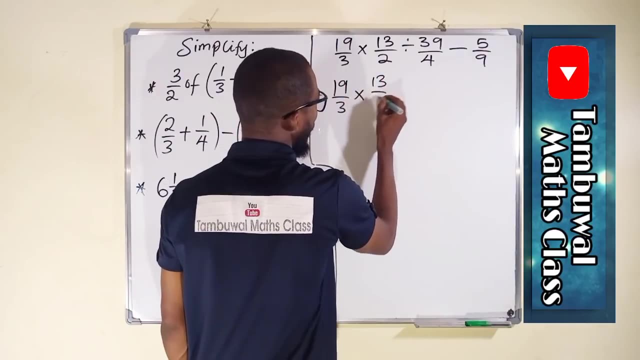 But remember, division can also be converted into multiplication by taking the reciprocal of the next term there. So this becomes 19 over 3, multiplied by 13 over 2, multiplied by then you take the reciprocal, we have 4 over 39..